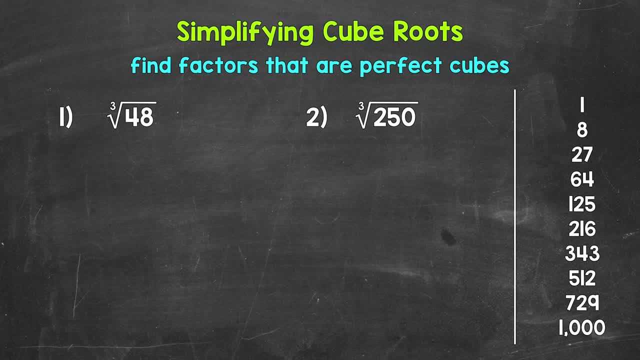 Now to the right. I have the first 10 perfect cubes. Knowing and being familiar with these, or as many of these as you can, will make simplifying cube roots and working with cube roots in general much easier. So are any of the first 10 perfect cubes? 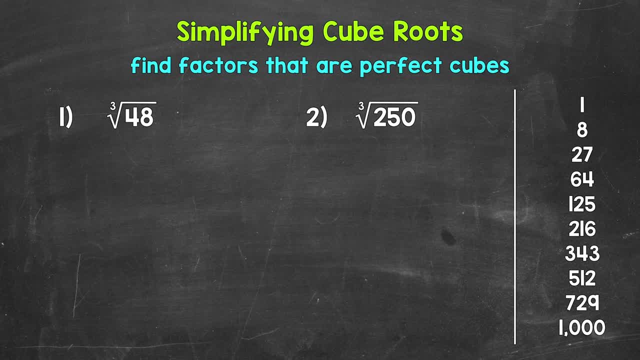 Are any of the first 10 perfect cubes a factor of 48?? Yes, 8 is a factor of 48. We know that 8 times 6 equals 48.. 8 and 6 are factors of 48. They go into 48,, so to speak. 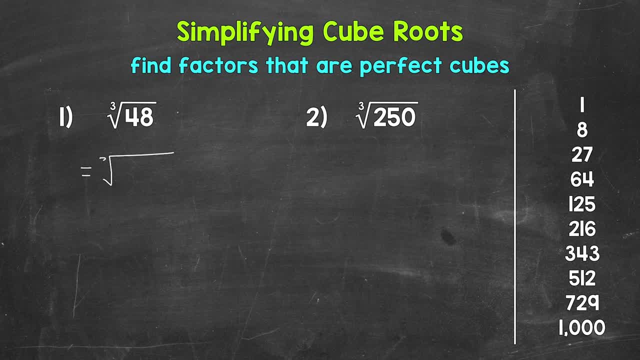 So let's rewrite the cube root of 48 as the cube root of 8 times 6.. Now the multiplication or product property of cube roots. lets us see how to simplify cube roots. Let's split this into the cube root of 8 times the cube root of 6.. 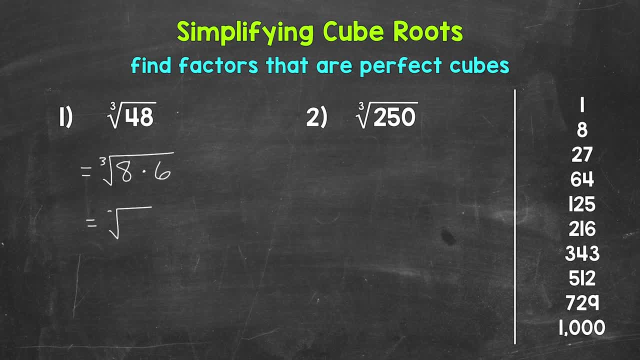 Meaning we have the cube root of 8 times the cube root of 6.. This is still equivalent to the cube root of 48. We're not changing the value of anything at all. Now we can take the cube root of 8,, which is 2.. 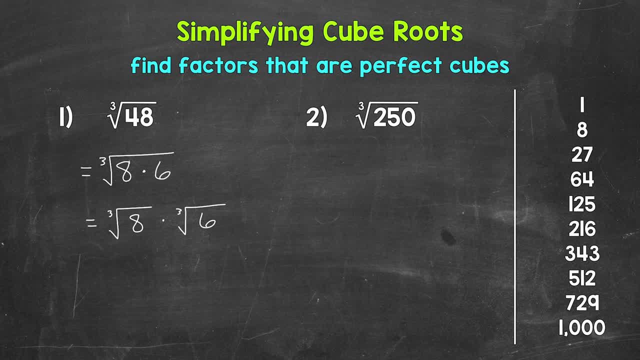 2 times 48.. 2 times 2 equals 8.. So again, the cube root of 8 is 2.. So we end up with 2 times the cube root of 6.. And that's our final simplified answer. 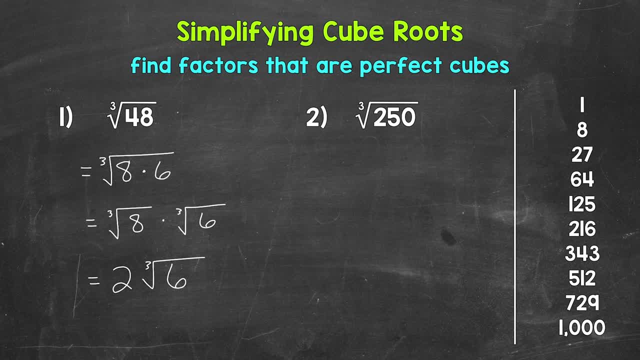 We can't simplify or break this down any further. So again our final simplified answer: 2 times the cube root of 6.. Let's move on to number 2, where we have the cube root of 250.. 250 is not a perfect cube, but we can simplify. 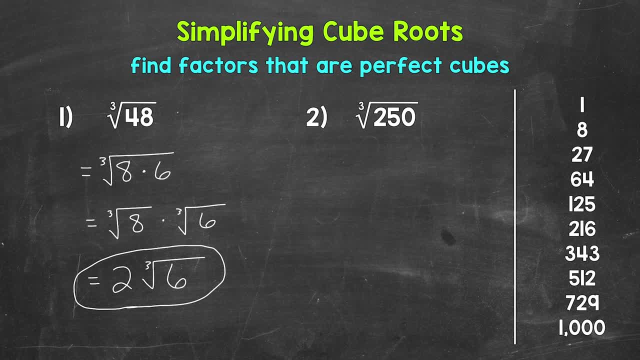 We need to look for factors of 250 that are perfect cubes. Well, 125 times 2 equals 250, and 125 is a perfect cube. Since there's a factor of 250, that's a perfect cube, we can simplify.